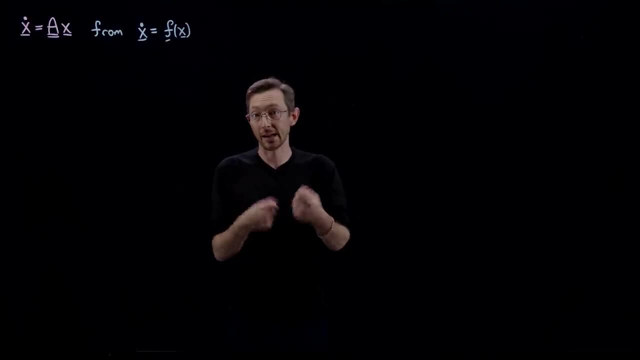 eigenvalues, some where we have one unstable and one stable saddle points, and also systems where we have complex conjugate eigenvalues, systems that kind of oscillate or rotate in time. But most of the real world is not linear. Most of the real world is not, you know, small angle. 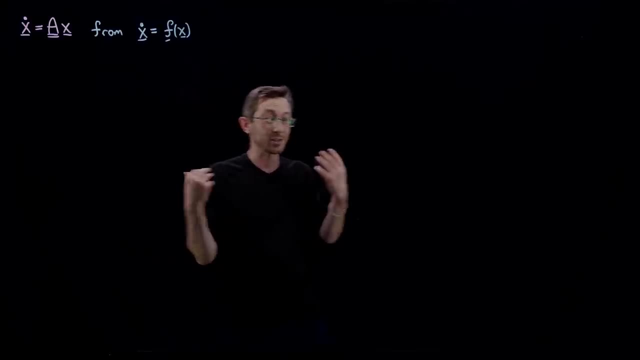 approximations of a pendulum and things like that. Most of the real world is actually non-linear. When you think about Newton's law of gravitation and planetary dynamics, or an actual pendulum has, you know it's not theta. double dot equals theta or minus theta. it's minus sine of theta. There's non-linear. 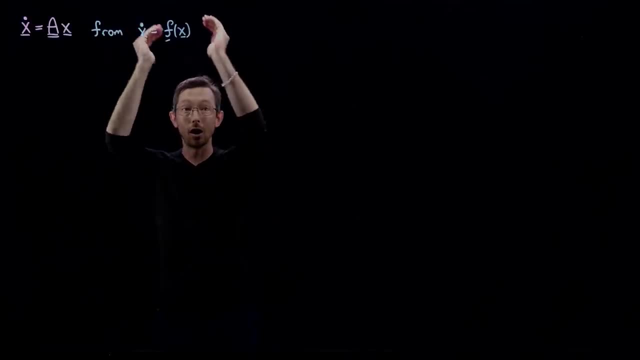 terms, And so what we're going to talk about is how to analyze honest to goodness, fully non-linear differential equations that are really nasty, by finding fixed points and linearizing, zooming in near that fixed point where it looks. It's approximately like this system, where we have tools where we can analyze that system. So this is one of my 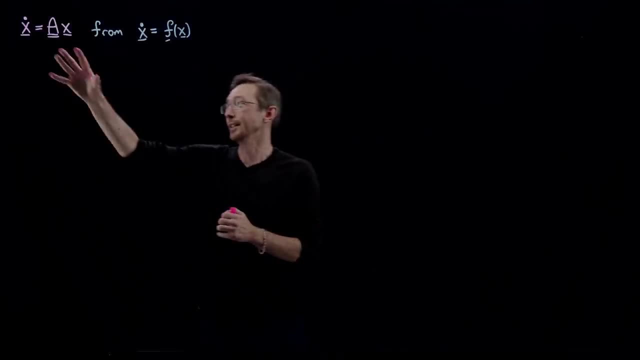 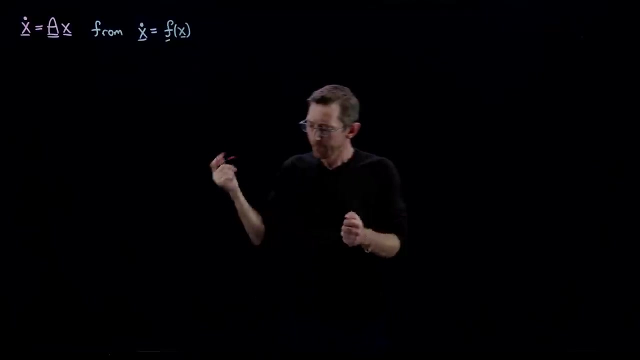 favorites. This is really a big step, transitioning from kind of intro, simple linear, ordinary differential equations to starting to build the framework and the scaffolding and the architecture for solving this. you know much, much richer class of very non-linear systems. So specifically this is called linearizing, or 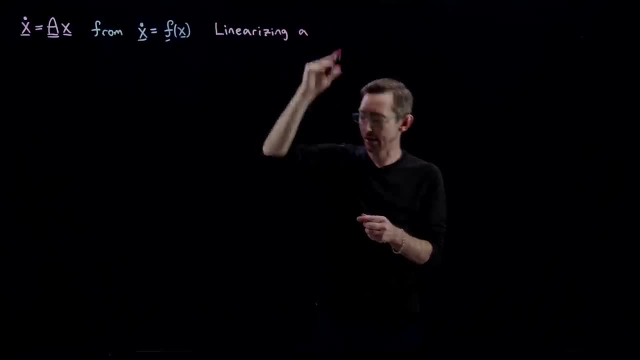 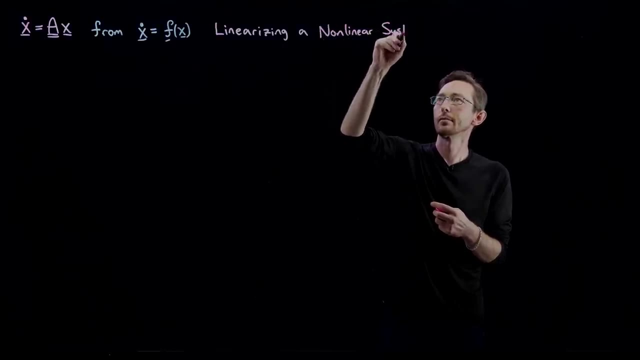 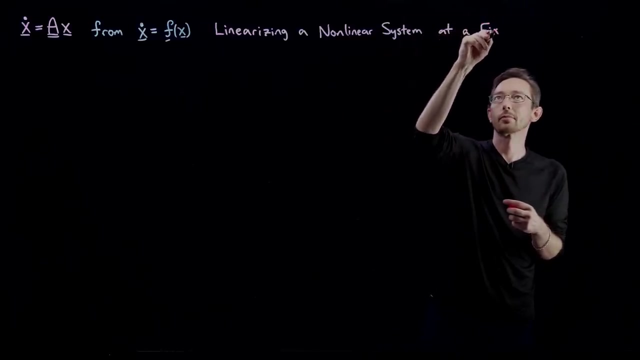 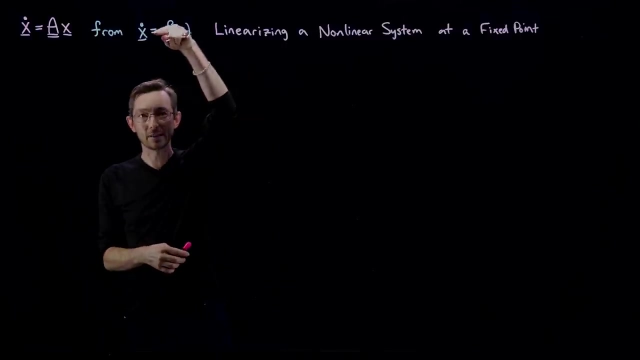 linearization, linearizing. So I'm going to define a non-linear system, non-linear system at a fixed point. So I'm going to define all of these terms at a fixed point. And one of the reasons that non-linear systems are difficult is because linear superposition doesn't necessarily hold up here for a non-linear system. 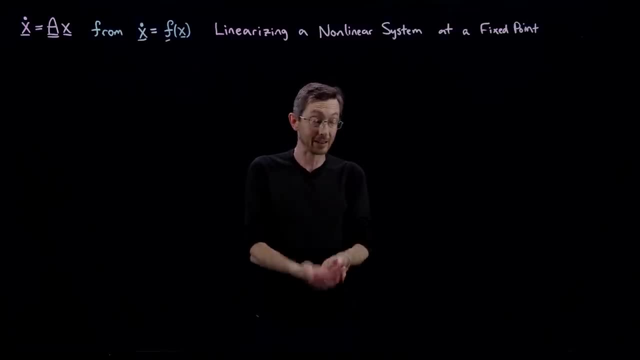 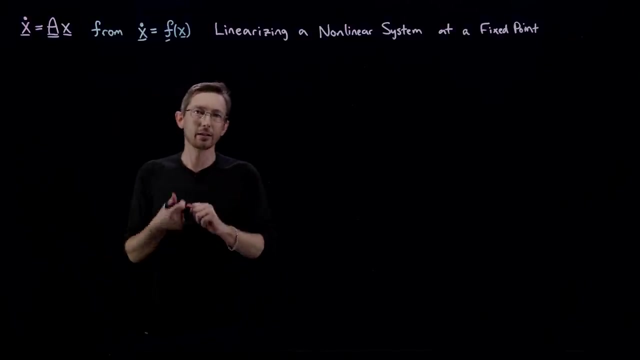 I can't take different solutions and add them up and expect them to still be a solution, Like I can with these linear systems. So we need fundamentally different techniques to solve these. So what we're going to do is start with a generic non-linear system. X dot equals F of X. 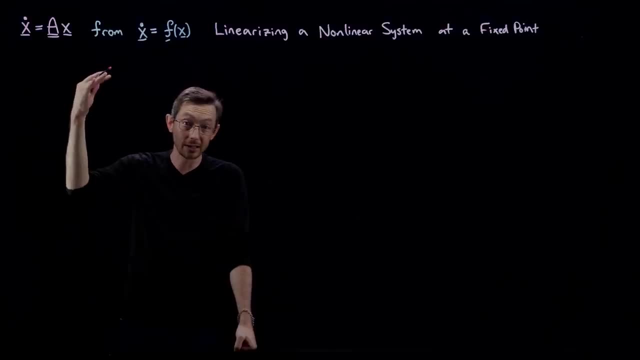 And I think I'm going to drop the underbar. Just assume that these are vector systems. These are, you know, X is a vector of states And this is a system of differential equations. Remember earlier, you know, X could have been the populations of the. 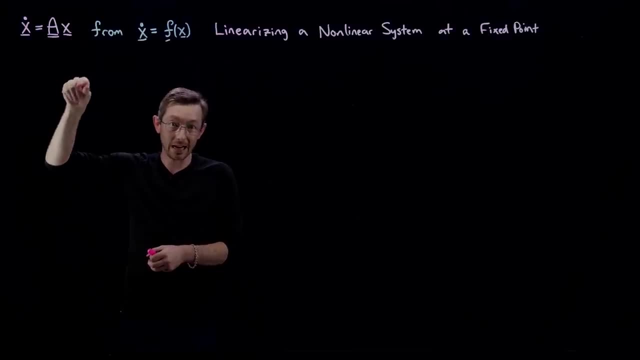 bunnies and wolves and cats and dogs and tigers and whatever, like a bunch of animals, And it was linear and diagonal and decoupled if they were all in different compartments in a zoo. But if I have them in the wild in the wilderness now, those animals are eating each other and doing all kinds of you know there's interactions. 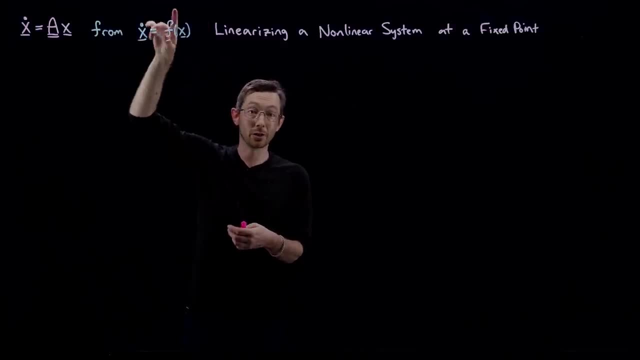 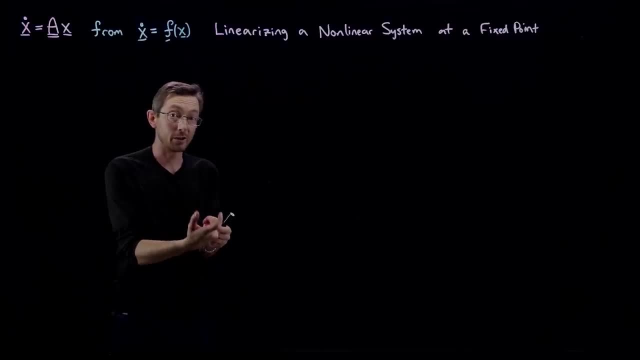 the number of bunnies that get eaten by wolves is not just proportional to the number of bunnies, It's proportional to the number of bunnies times the number of wolves. That's a non-linear term in this differential equation. OK, so X dot equals F of X. 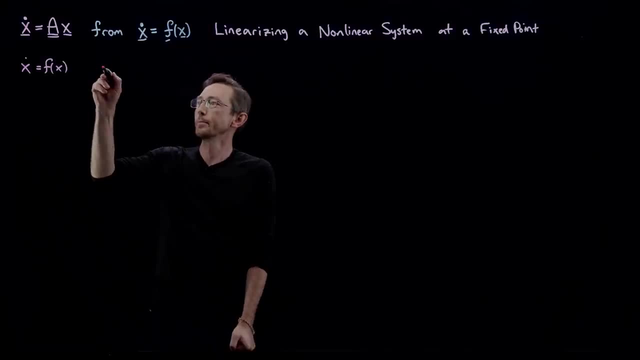 We're going to say that this has a fixed point. X bar is a fixed point Literally means that it stays put. It stays fixed at that point. If you start at X bar, you stay fixed at that point. It's a fixed point if my function F, evaluated at X bar, equals 0.. 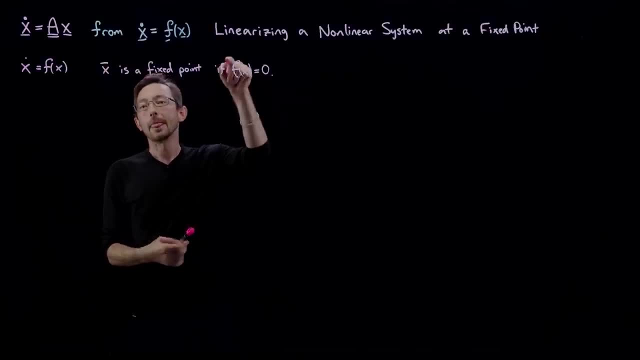 That's kind of a funky F. Sorry, it looks weird. That's an F. If my function evaluated at X bar equals 0,, then that means that d dt of X is 0 at that point, meaning that it doesn't change in time. 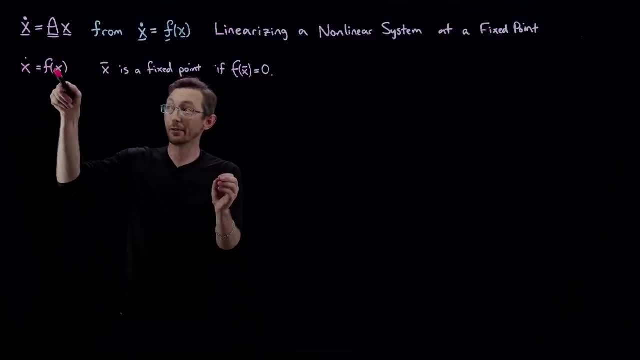 There's no dx dt because F of X bar equals 0.. If I start at this point, I stay at this point, because it's fixed, because there's no change in time from that point. Good, In a word, d dt of X bar would be 0.. 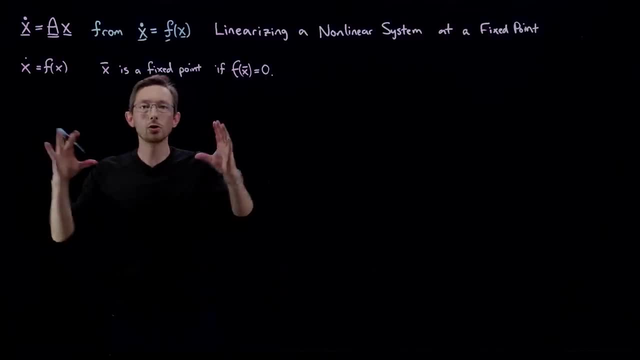 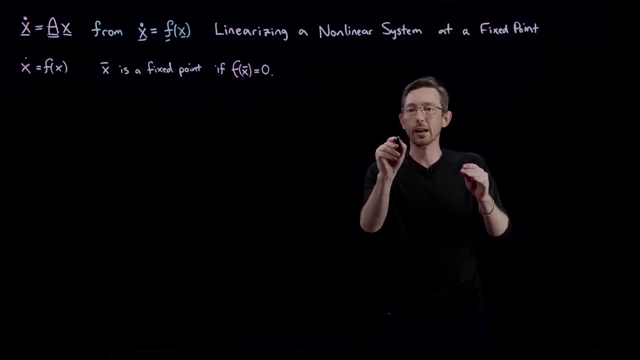 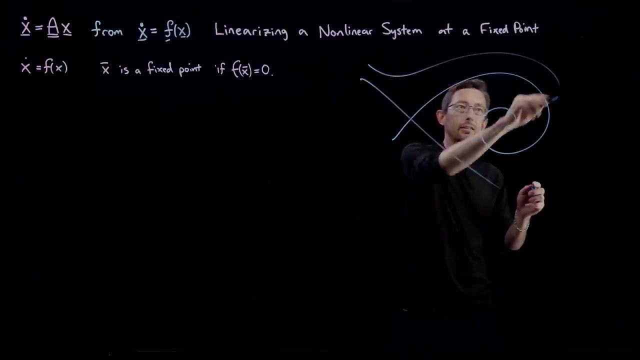 What linearization does is that we zoom in to a neighborhood near that fixed point. I'll draw a little picture here. I'm actually going to show you this example later- where, in two dimensions maybe, I have some dynamics that look like this: 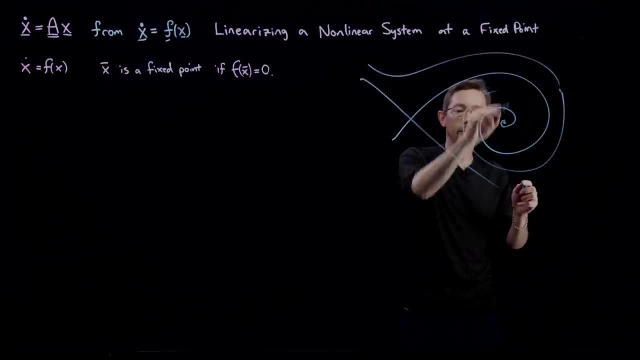 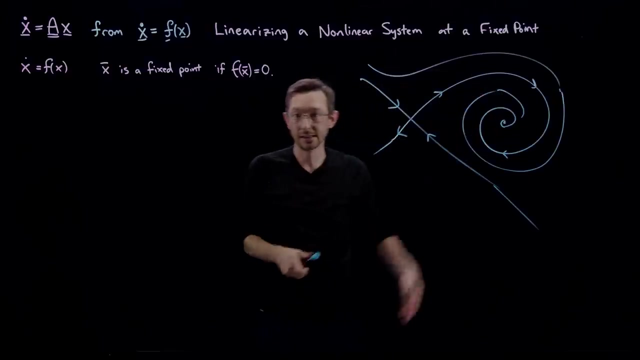 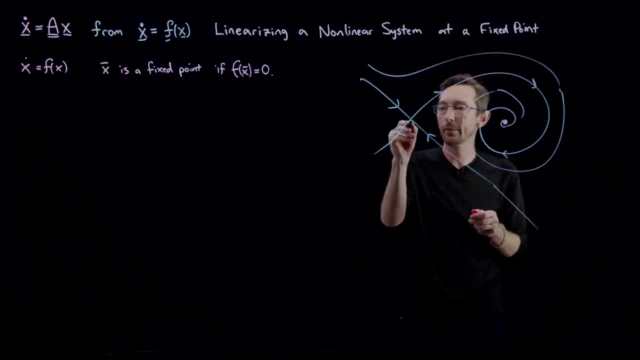 I'm trying to think of how to actually draw this. Maybe I have some system that looks like this. I've got all this nonlinear stuff. I've got lots of trajectories in this system, but I have a couple of fixed points. I've got one of them here and I've got one of them here. 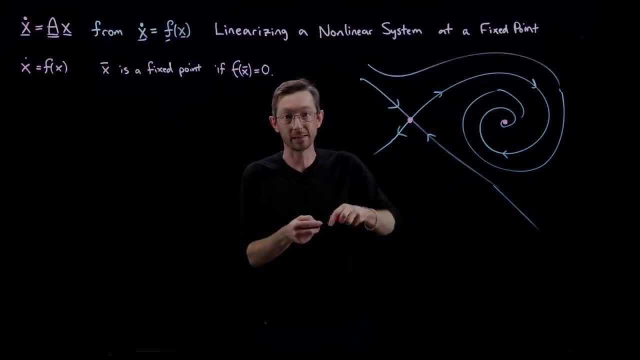 If I started exactly near that fixed point, or exactly near that fixed point, I would stay put there forever. What we're going to do is we're going to zoom in on one of these fixed points. We're going to zoom in on a little teeny window around here. 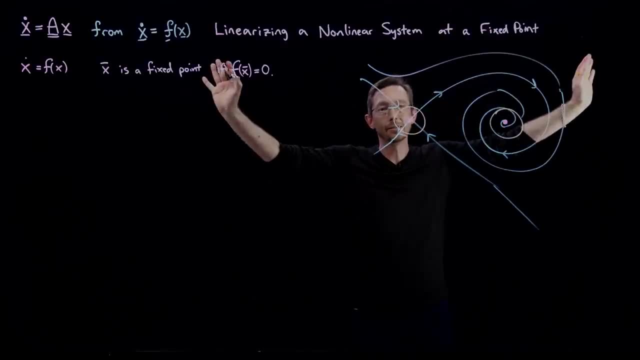 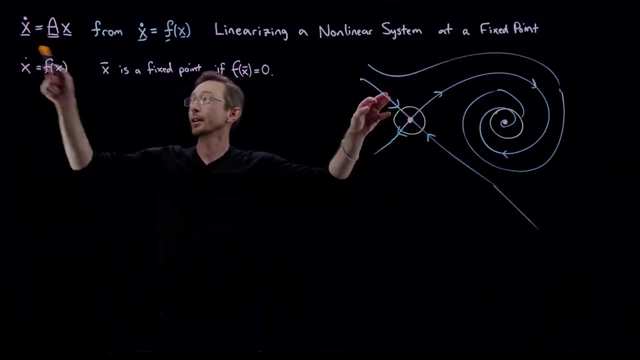 or a little teeny window around here, We're going to pretend that nothing else exists. We're just going to zoom in to this little neighborhood. around these fixed points, In that little neighborhood, they're going to look like linear systems that we know how to analyze. 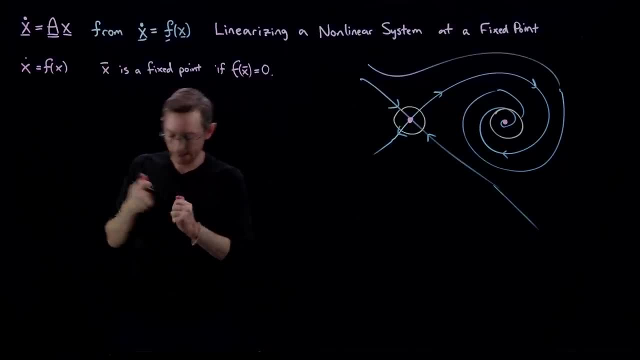 This is a fixed point. Now what we're going to do is we're going to say, for some point, x that is near that fixed point, nearby to that fixed point. Basically, we're going to say that x equals x-bar plus a little delta x. 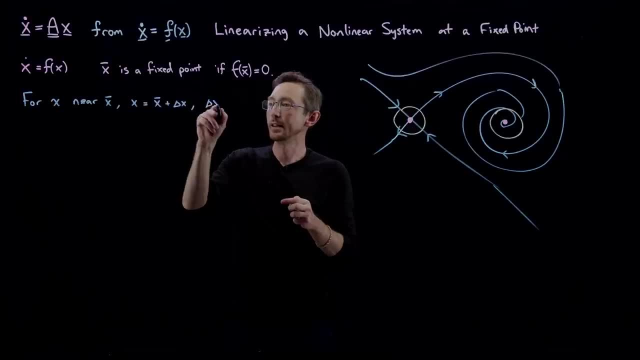 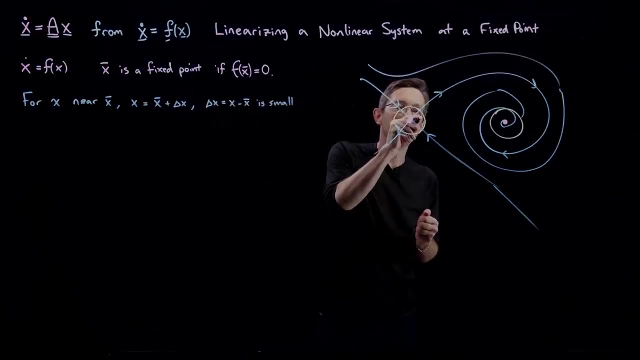 where delta x is small, Delta x equals x minus x-bar is small. I'm just going to keep going back to this little picture to help orient myself If I'm at this little point. this is my point x and this is my point x-bar. 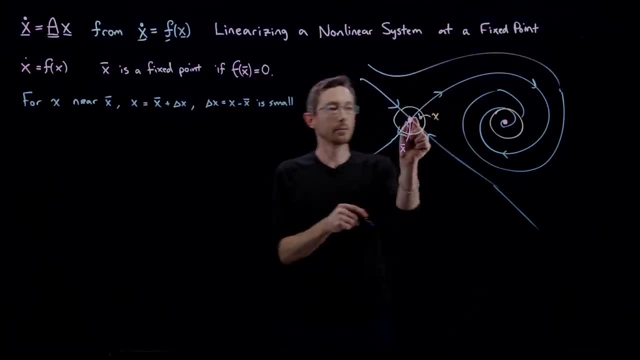 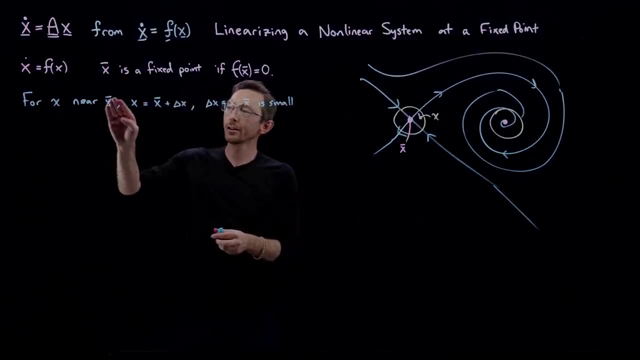 and this little difference between them, this little delta x here, this little delta x distance. that's a small distance because we've zoomed into a small neighborhood For x near x-bar, meaning that it's a little small delta x apart. 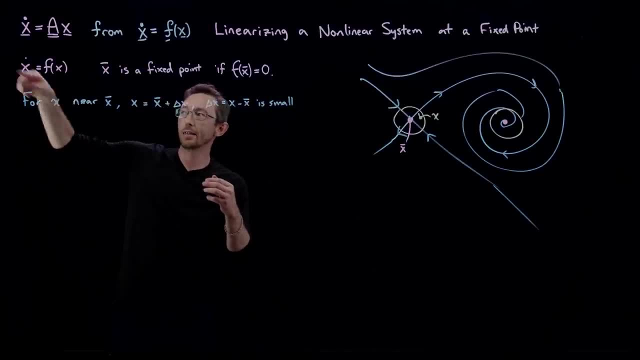 then we can tailor expand this differential equation. This is where it gets interesting. We can tailor expand this differential equation and we get. how do I want to write this? I want dx, dt equals f of x. Good, I'm just convincing myself that this is true. 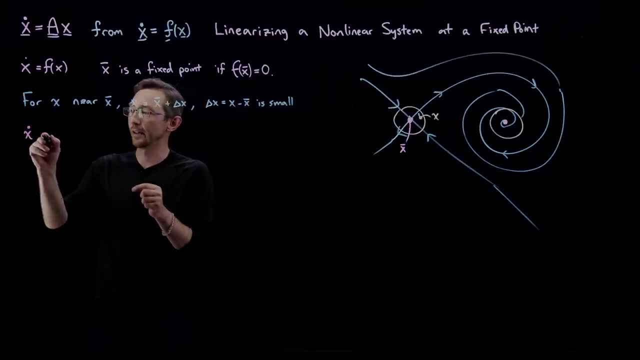 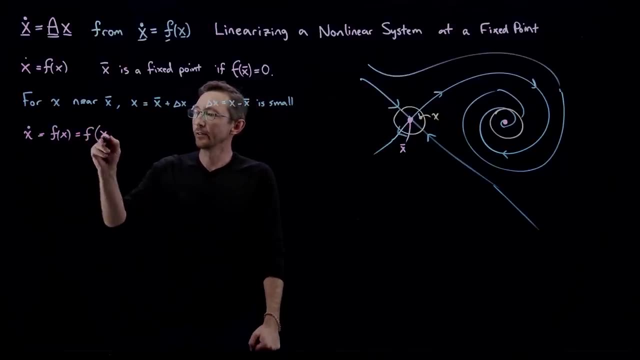 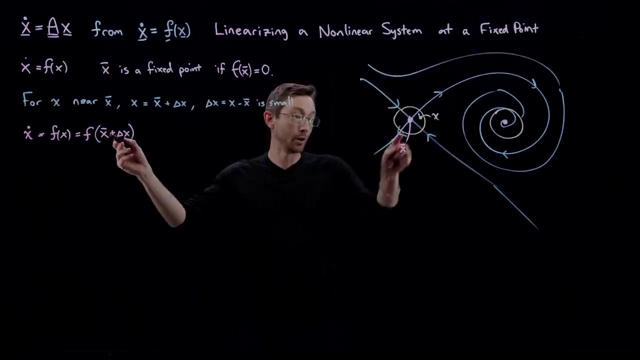 x-dot is of course going to equal f of x. That equals f of x. That is going to equal f of x-bar plus delta x. Because delta x is small, I can tailor expand at this base point x-bar at my fixed point in powers of delta x. 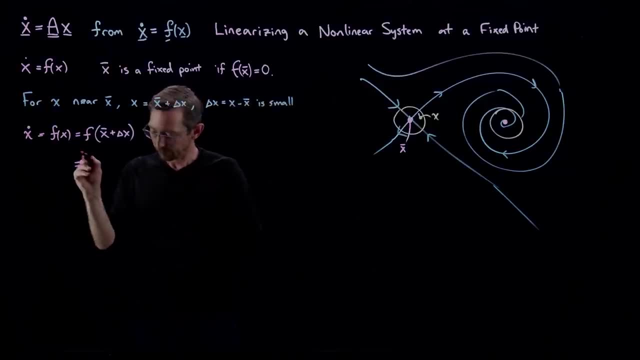 That's pretty easy. That's going to equal f at x-bar, plus the derivative of f with respect to x, Because x is a vector and f presumably has multiple components. also, This is literally, let's say, x1, x2, dot, dot, dot, xn. 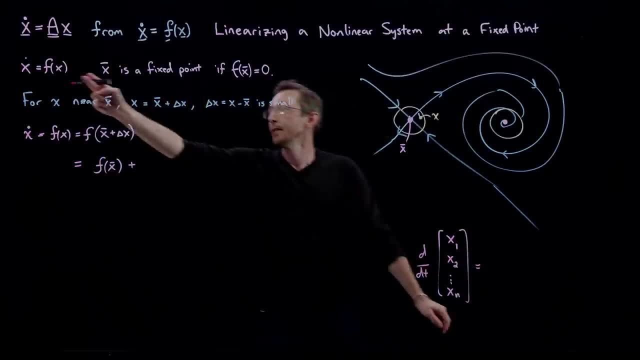 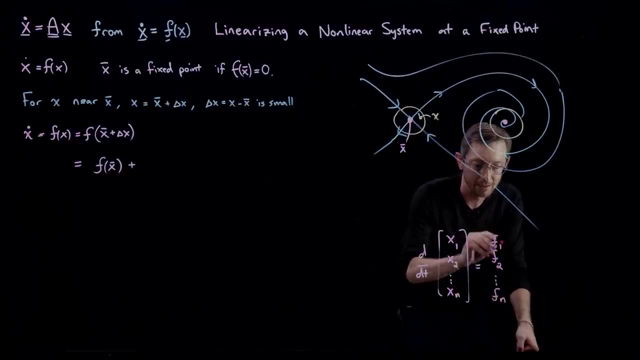 d, dt of that equals, Then this f also has components. It has f1, f2, dot dot dot fn. These are all functions of x1, x2, dot dot dot x1, x2, dot dot dot x1, x2.. 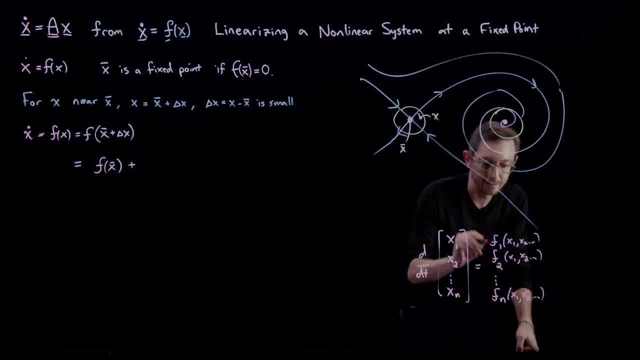 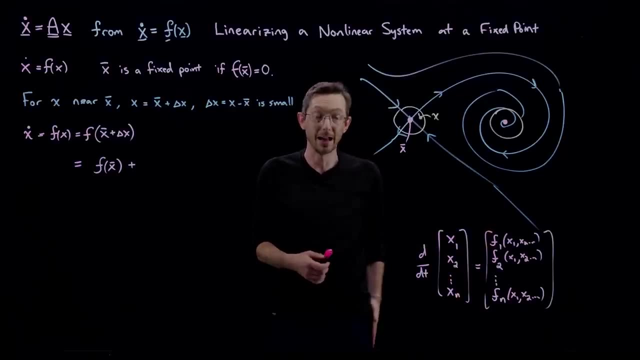 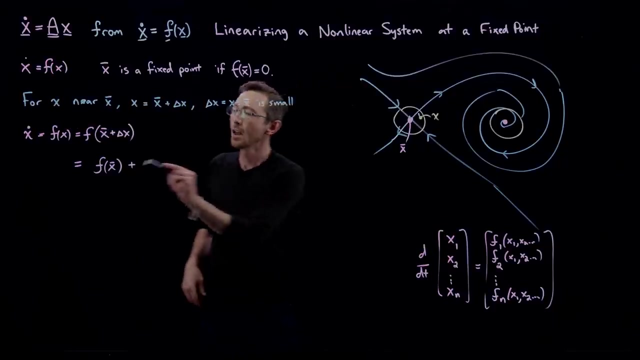 This is literally a vector-valued function. There's components to this function: f, One for the x1-dot equation, one for the x2-dot equation, one for the x3-dot, and so on and so forth. When I compute the derivative of f with respect to x, 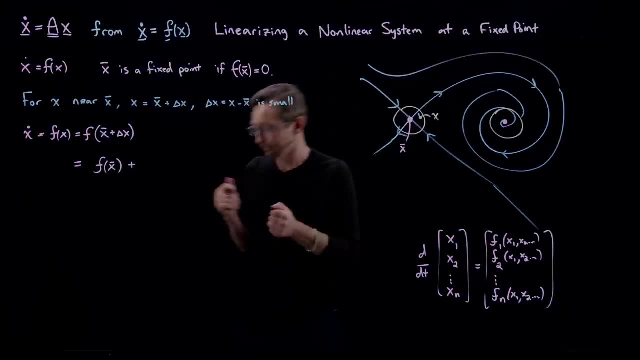 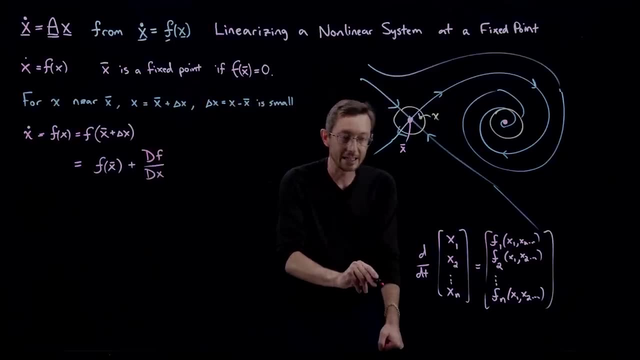 this is actually a matrix derivative called a Jacobian. Usually we write it with a big capital- D, f, dx- Instead of little df, little dx. this is big df, big dx, because that means I'm going to take a matrix of derivatives. 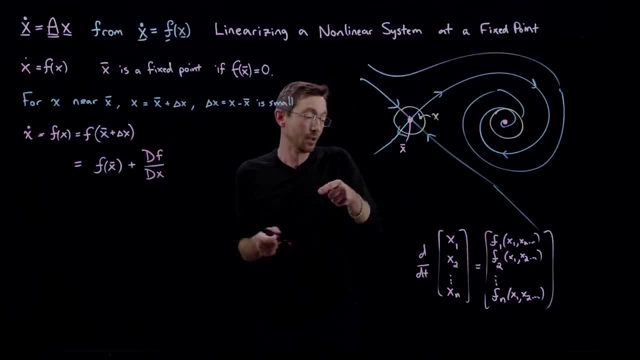 I'll show you what this means in a minute, but it's a matrix of partial f1, partial x1, partial f1, partial x2, partial f2, partial x1, and so on and so forth. This is a matrix of derivatives that I evaluate at x-bar times. 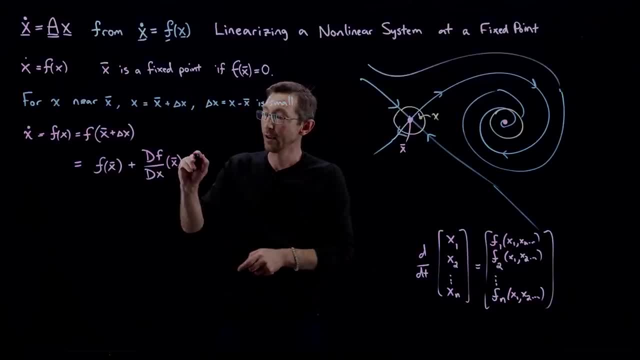 this is literally a dot product, because this is a matrix dotted with delta x- I'm sorry, I don't even need parentheses here- Dotted with delta x, because delta x is also a vector. This is like a vector: delta x. 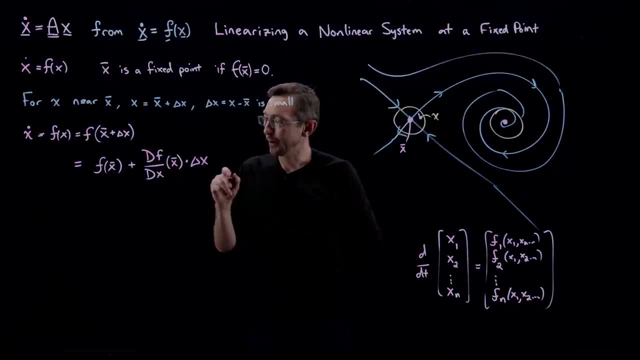 That's the first term in my Taylor series, plus the second Jacobian derivative, the second matrix derivative of f with respect to x-squared, evaluated at x-bar, again dotted with delta x-squared plus cubic quartic, and so on. 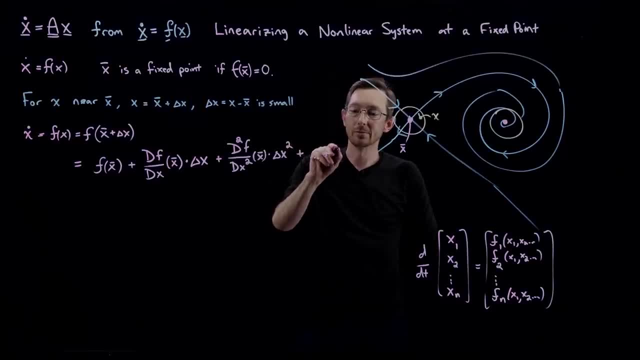 plus dot, dot dot, forever and ever and ever. and sometimes we just say plus higher order terms. This goes on and on. or plus order, delta, x, cubed and higher, That's another way to write it. This is the Taylor expansion of my dynamics. 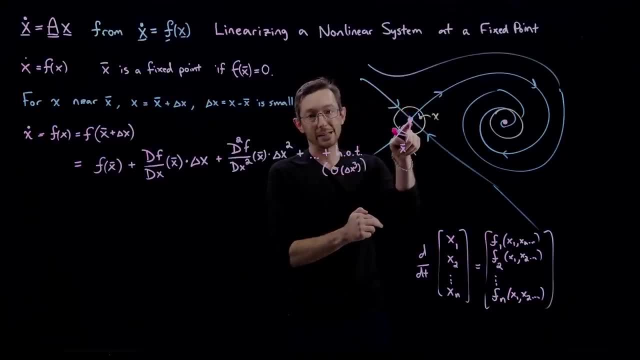 my nonlinear dynamics zoomed in around a fixed point- x-bar- where I'm only kind of a little delta x away from that fixed point, And so the key observation here is that all of these terms are very small, very small, very, very small. 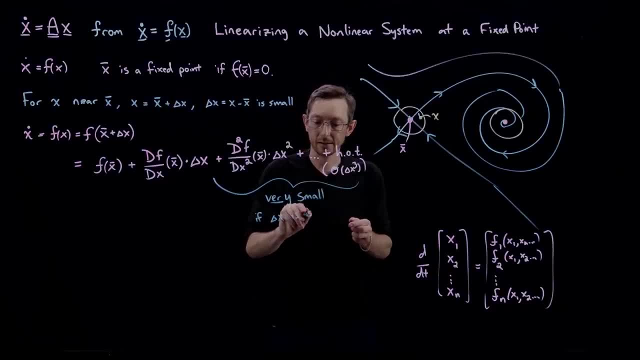 if delta x is small. So if delta x is small, then delta x-squared is tiny and delta x-cubed is minuscule, and delta x to the fourth might not even be there. It might as well. And all of these terms. 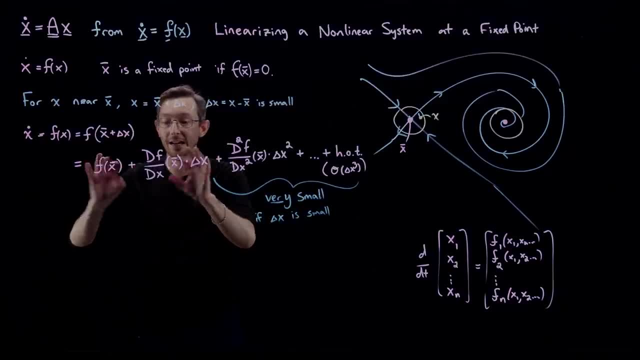 kind of are approximately zero, And so you get a very good approximation of the dynamics with this term here. And then the last piece is, of course, f of x-bar is equal to zero. So this is kind of the only term that's left in the dynamics. 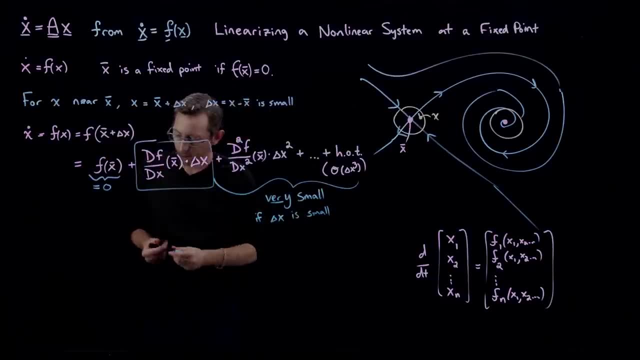 when these are small and this is zero. And so what we have is that basically, and of course, x. here we have that basically, x-dot is really ddT of x-bar plus delta x, But x-bar is just a number, It's like a constant vector. 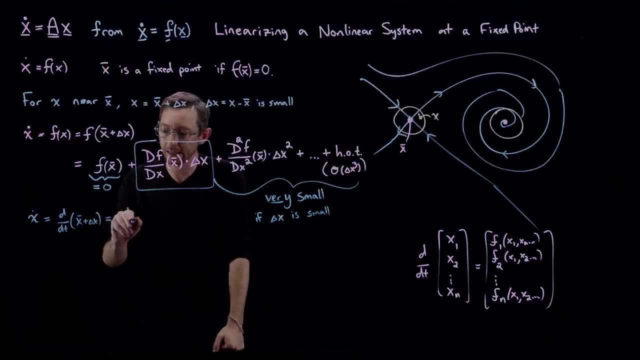 at that fixed point. And so really this is like ddT of my delta x. So delta x is kind of the new state of my system zoomed in here. ddT of delta x equals this Jacobian matrix: df, dx evaluated at x-bar times. delta x. 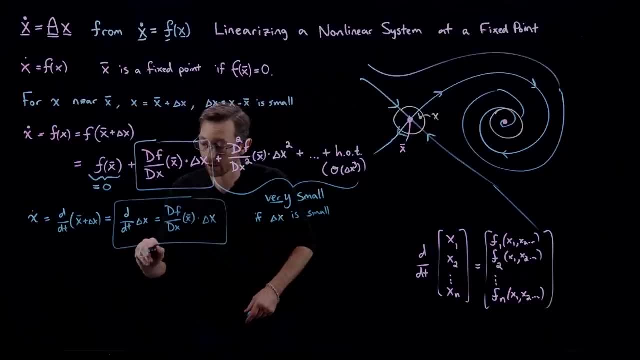 And I claim that this is going to be a linear, ordinary differential equation: linear ODE in delta x. And now I'm going to show you how to compute these df dxs, what these mean and why this is linear. Okay, Good. 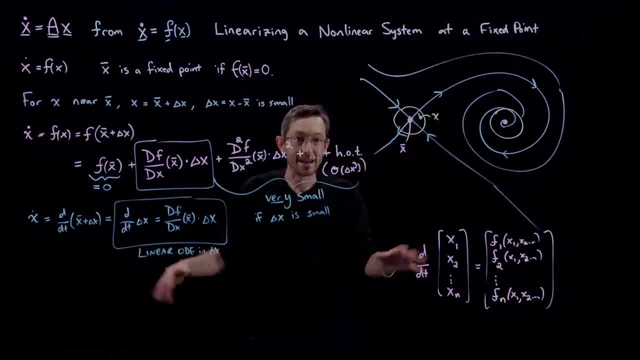 So this was about a big step. Now, what I'm going to do is I'm going to show you how to compute these matrix, these matrix derivatives. Maybe I'll just do it for a 2x2 f vector field, because it'll be a lot easier. 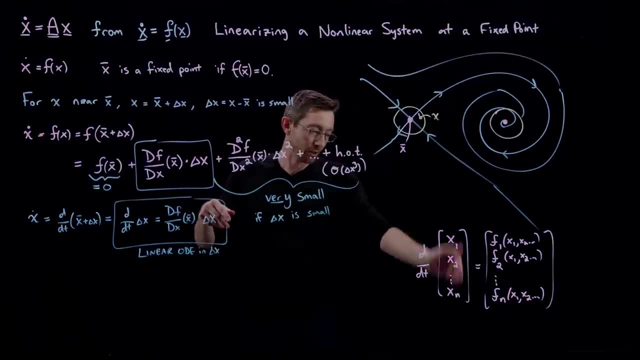 but it's very, very simple to generalize this for an arbitrary n degree of freedom system. you know a vector where x has n elements. Okay, So good, I'm going to write that out for you, just so that you see. So. 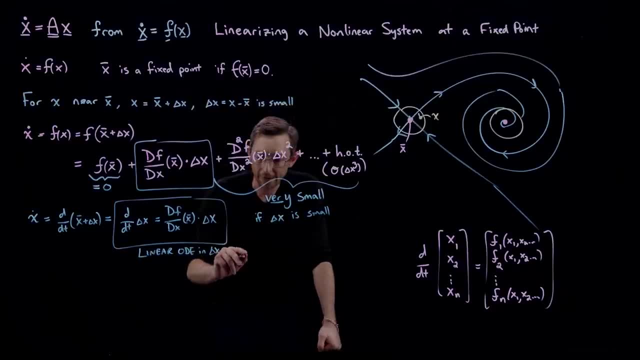 and I think I'm actually going to write it right here. So this df, dx, and you know what, I'm actually going to write it in general because I want to. Okay, I'm going to write it in general and then I'm going 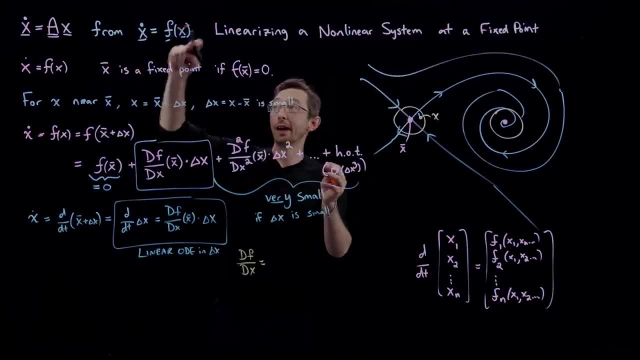 to give you a 2d example, like an actual f of x in 2d, like this: and we're actually going to pick a fixed point and linearize. So that's how I'm going to end this. So df, dx for an arbitrary. 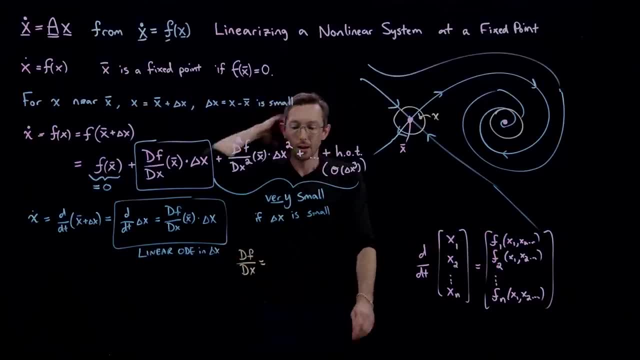 you know n degree of freedom system is going to be a matrix of partial derivatives. It is going to have partial f1 with respect to x1,, partial f1 with respect to x2,, dot, dot, dot. partial f1 with respect to xn. 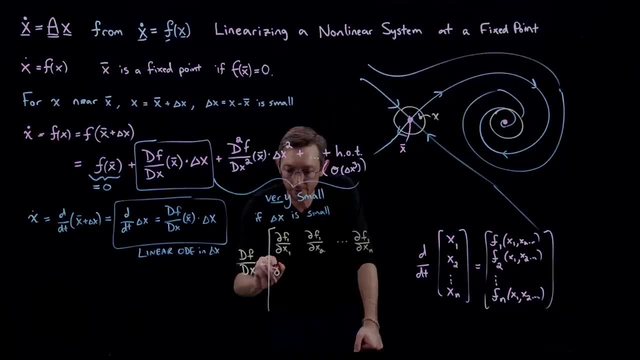 Okay, that's the first row of this thing. The next row, as you may have guessed, is partial f2, the second row partial x1, partial f2, partial x2, dot dot dot. partial f2, partial xn. 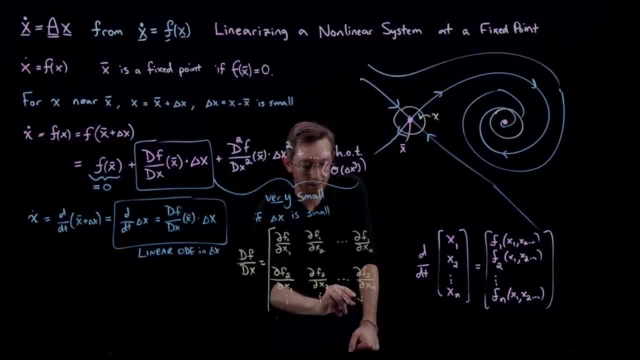 and then you know, dot, dot, dot, dot, dot, dot. every row is the same. And then the last row is partial fn. partial x1, partial fn, partial x2, dot dot dot partial fn. partial xn. 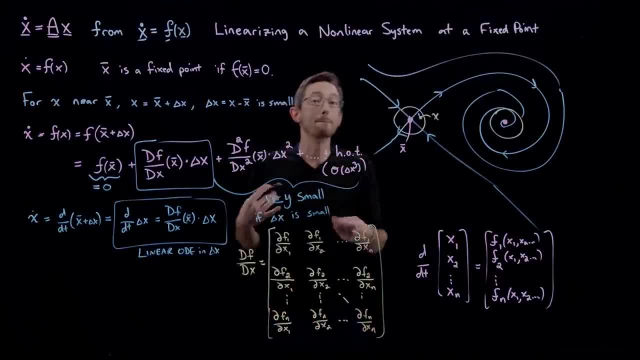 and that is literally my matrix of partial derivatives. my this is df, dx, this is called the Jacobian matrix. very, very important. And here we are. these are all functions. now, these were functions, and so their derivatives are functions. 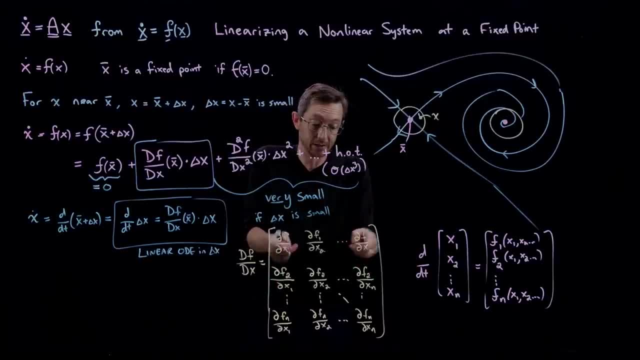 And here we're going to evaluate this. this is a matrix of functions. Here we're going to evaluate this. at our fixed point, x bar, and this is going to turn into a matrix of numbers. These are all going to be numbers when I plug in x bar. 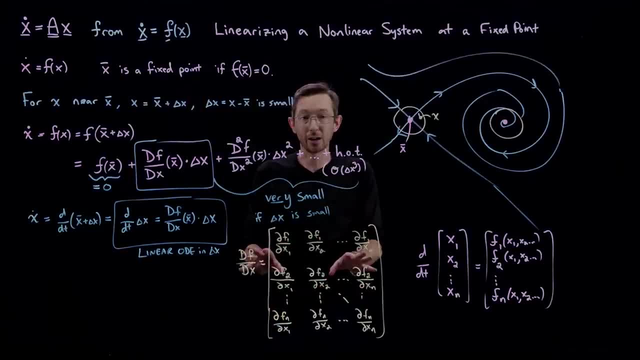 into all of these equations. Okay, So that's what I mean by df, dx. This is literally a matrix, and that's why this is a linear ODE, because it looks like x dot equals ax, with this being the A matrix. 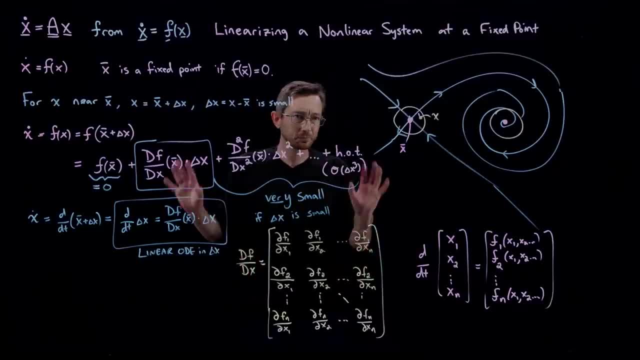 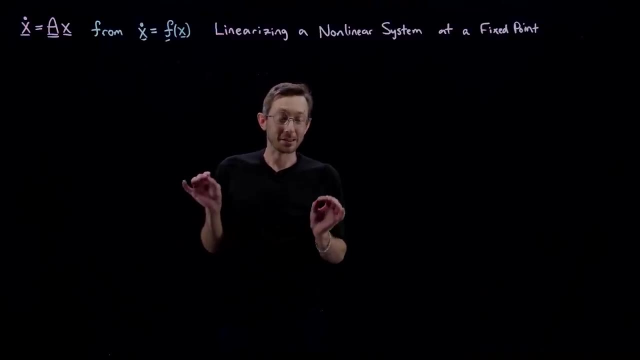 Okay, good, I am going to erase some stuff and then we're going to write down a two-dimensional example and solve it. I wish erasing that was as easy in real life. Okay, so the example we're going to do: 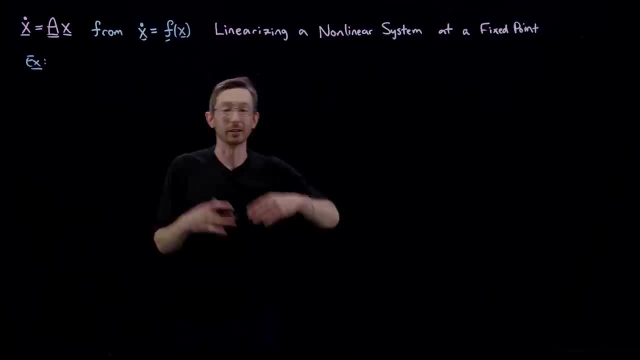 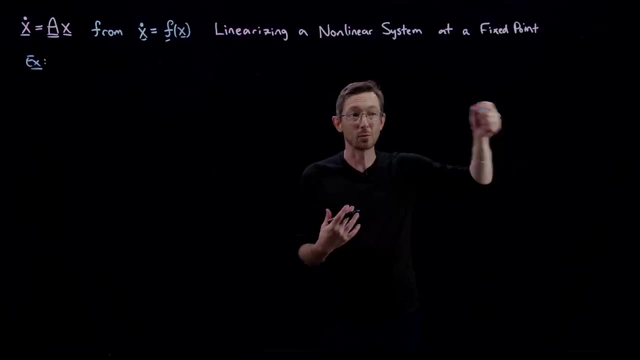 this is a really simple example and I'm going to actually, in the next few lectures, build up a bunch of examples, some of my favorite examples from Newton's second law: f equals ma. We're going to look at potential systems where we literally take like 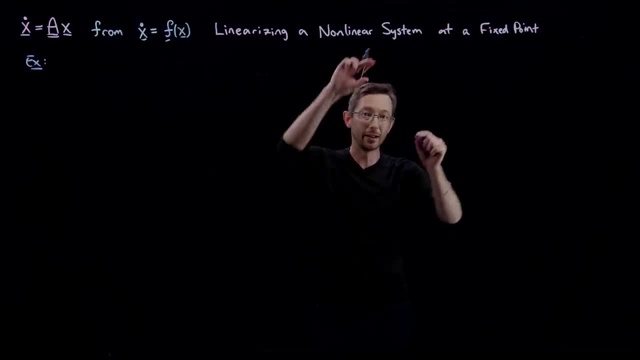 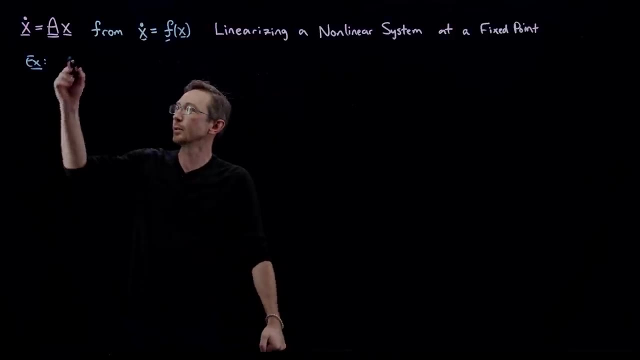 some potential function and we put like a bead, you know, on that potential function and watch it move. We're going to do a bunch of examples, So in this one what we're going to have is f of x and remember, f is a vector. 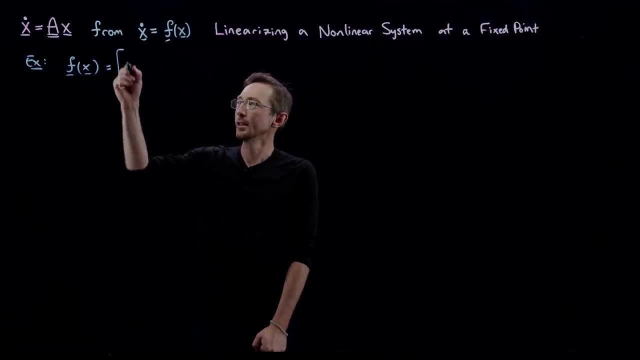 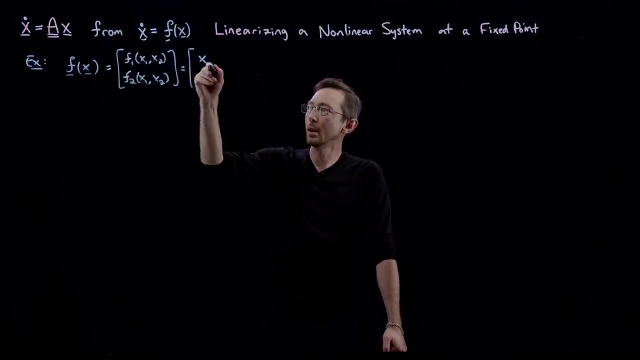 and x is a vector and of course you know that's f1 of x1, x2, f2 of x1, x2, and I'm specifically going to define these two functions to be x1 minus x1 squared. 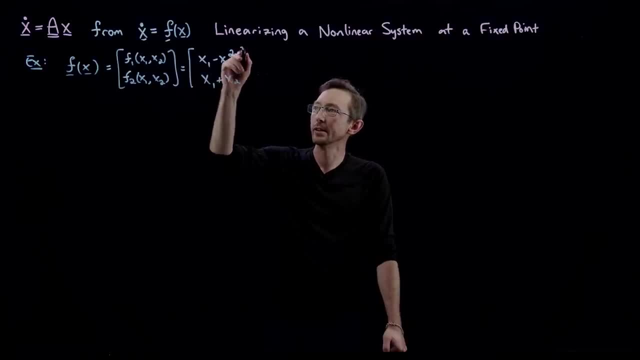 and x1 plus x2.. These are my f1 function and f2 function. I've chosen them to be easy on purpose because I want to make my life easy for this kind of introductory warm-up example, And for this example you can read these fixed points off: 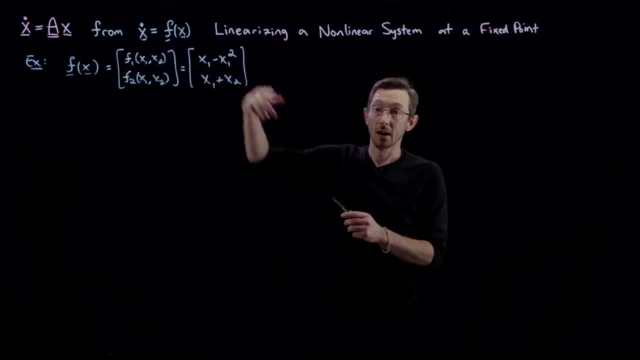 really easily. So there are two fixed points of the system where both of these equations are equal to 0. So in the top equation, x1, basically x1 can equal 0 or x1 can equal 1.. And if x1 equals 0,, 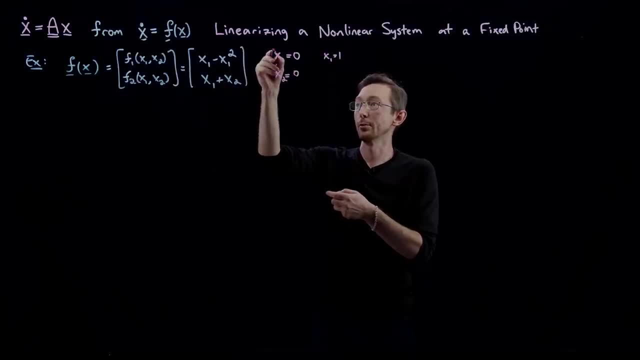 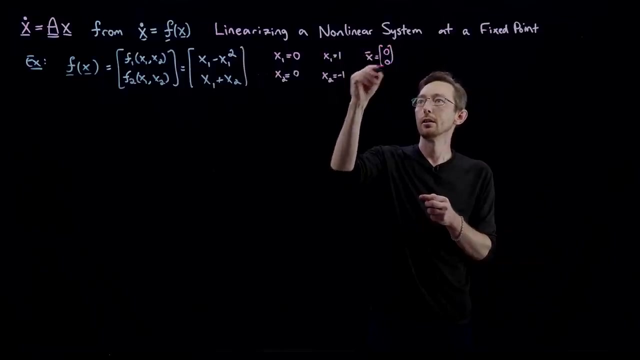 then x2 has to equal 0. That's a fixed point. And if x1 equals 1, then x2 equals minus 1.. So we basically have a fixed point. The fixed points x bar are 0, 0 and x bar equals 1 minus 1.. 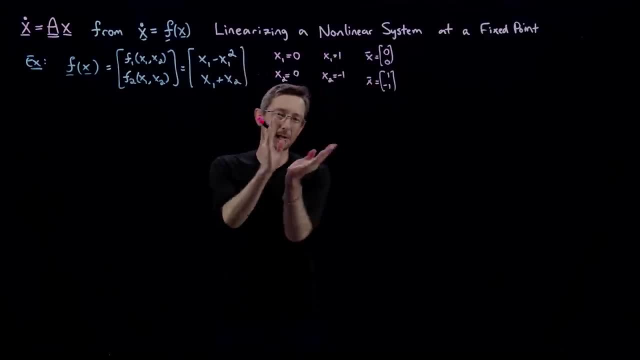 These are the two fixed points in phase space. I always call phase space the space of, you know, x1 and x2.. That's just an old habit. Okay, so the way that we basically linearize, so we want to zoom in. 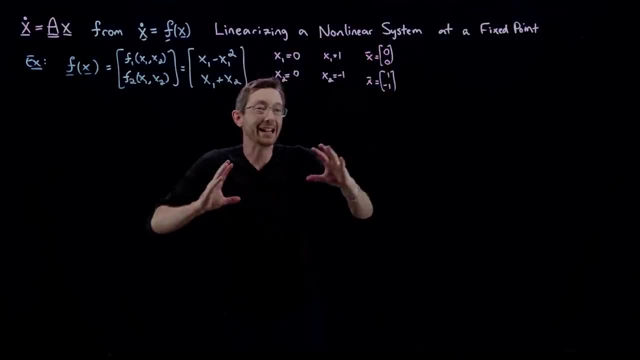 to a small neighborhood of these two fixed points And in that small neighborhood they're going to look linear, This nasty nonlinear system. you know, away from these points, all bets are off. But if I zoom in really close to the origin, 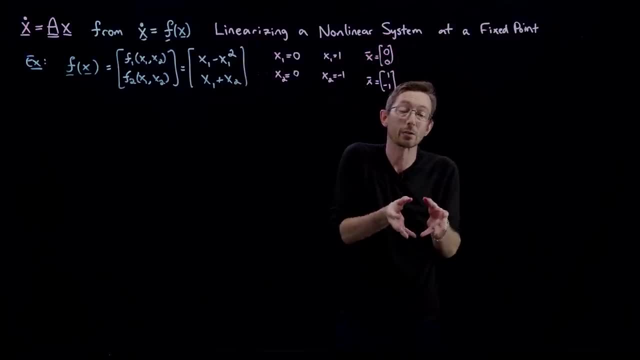 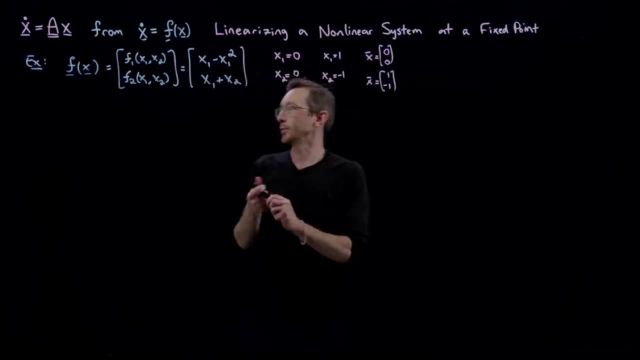 or really close to this point: 1 minus 1, the dynamics are approximately going to be linear according to that formula I wrote down before, And so I literally just have to write down this Jacobian matrix: df, dx, And that's my matrix of. 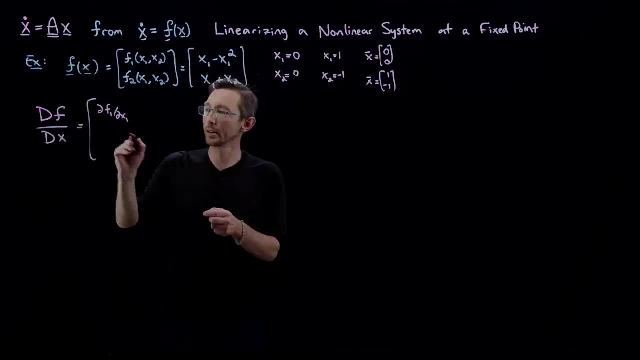 you know partial f1, partial x1, partial f1, partial x2, partial f2, partial x1, partial f2, partial x2.. I'm getting a little sloppy, you can see, But it's really easy. 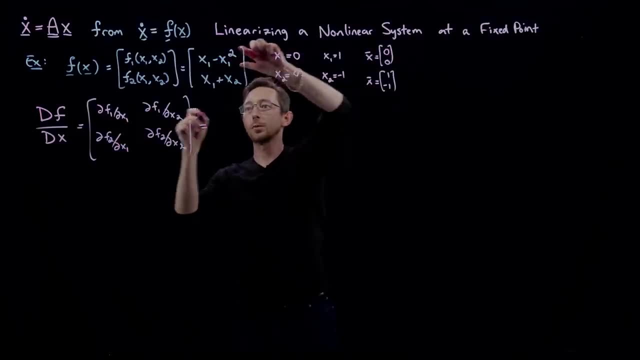 to compute these partials. So the partial of f1 with respect to x1 is 1 minus 2 x1.. The partial of f1 with respect to x2 is 0, because this has no x2s in it. The partial of f2. 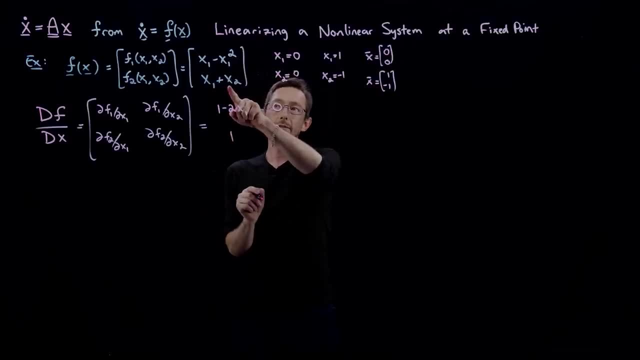 with respect to x1 is 1, that's really simple. And the partial of f2 with respect to x2 is also 1, that's really simple. So this is the Jacobian matrix in general, And now we have to evaluate. 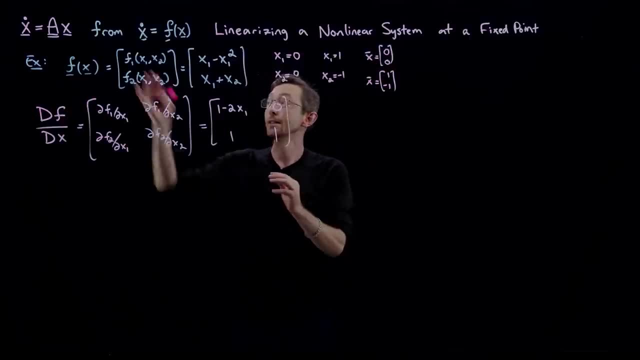 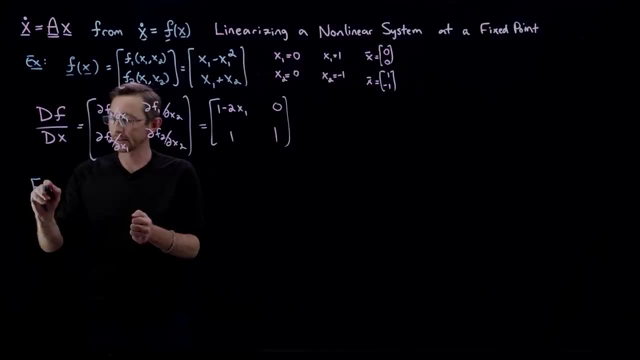 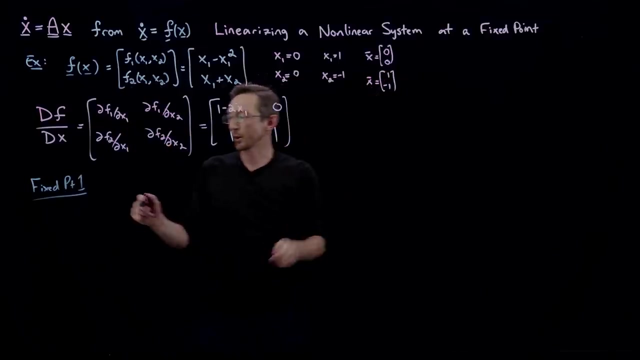 this Jacobian matrix at these two fixed points, to figure out what our A matrix is in those neighborhoods. Okay so, fixed point 1, let's say fixed point 2,. point 1, is, let's say, x-bar equals 0, 0,. 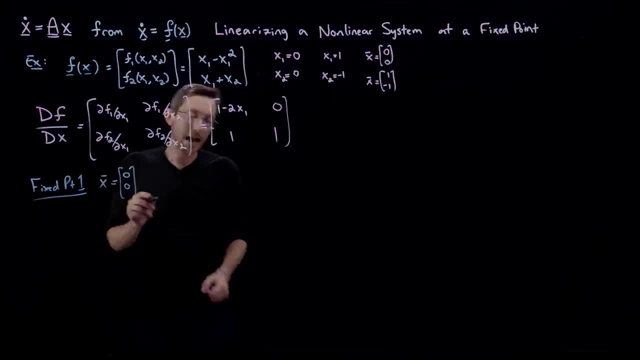 x-bar equals 0, 0. And so here what we have is df, dx evaluated at x-bar. We literally take x1 equals 0,, x2 equals 0, and we plug it in here And this matrix you know. anytime I see. 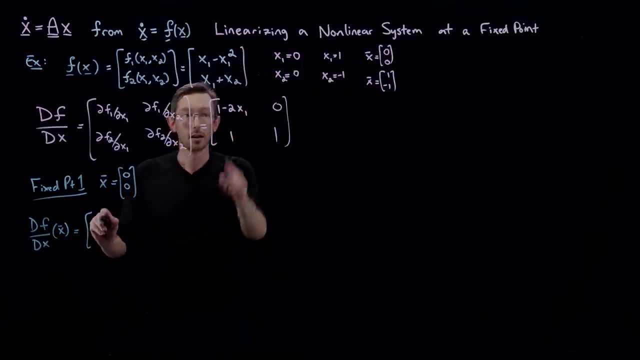 an x1 or an x2, they're equal to 0.. So this matrix becomes 1, 0, 1, 1.. That is the A matrix for my linearization. zoomed in at this 0, 0 point. 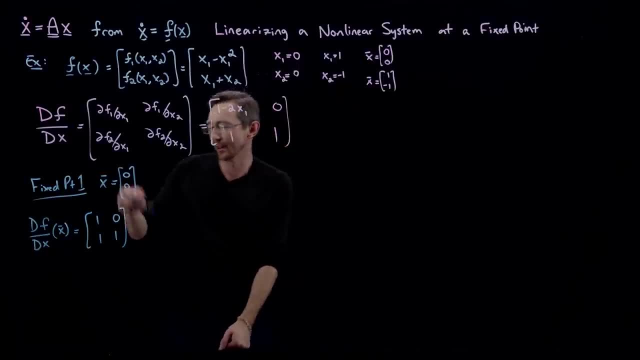 And we can do things like compute its eigenvalues. If I read these eigenvalues off, the lambdas are plus 1 and plus 1.. Any matrix that has zeros either above or below the diagonal, then the diagonal elements are going to be the eigenvalues. 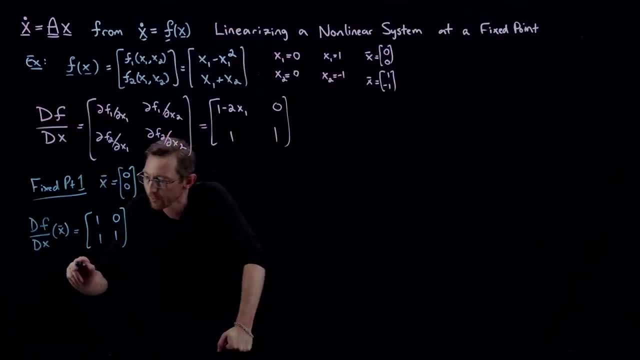 That's really easy to show. That's a good homework problem for you. And so the lambdas equals 1, 1.. So this one is unstable. It's like an unstable source. Okay, good, So that fixed point. things are going to emanate. 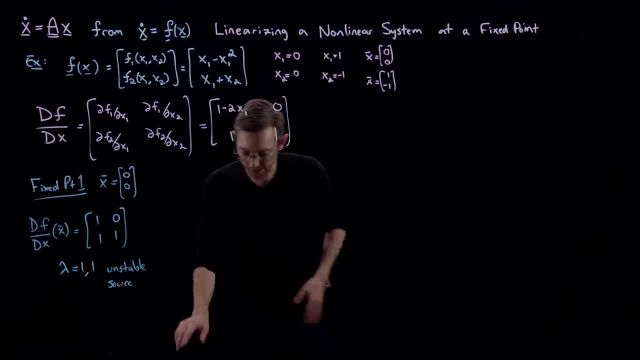 away from it locally in an unstable way. Let's look at my next fixed point. Maybe I'll do this one in orange. So fixed point 2, x-bar equals what was it? 1 minus 1.. Again, I'm going to compute: df, dx. 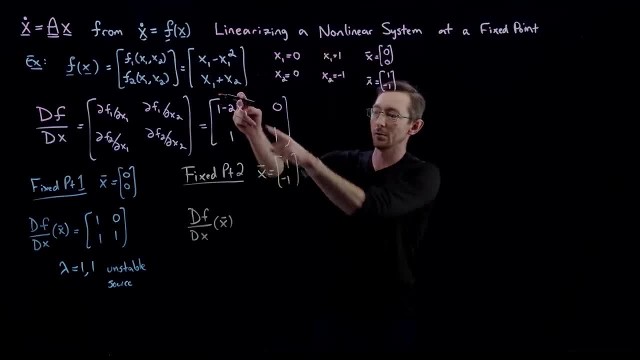 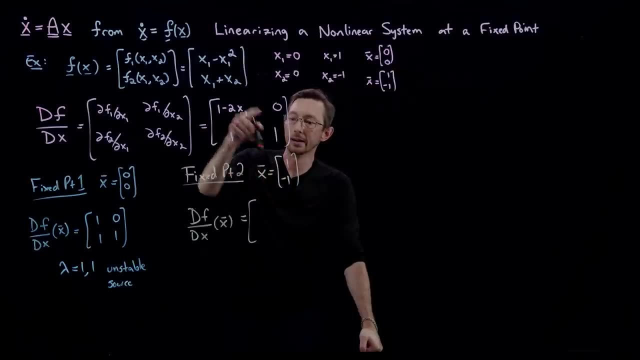 evaluated at x-bar, literally meaning I plug in 1 for x1 and minus 1 for x2, but there are no x2s here. So this Jacobian matrix is now 1 minus 2, is minus 1, 0, 1, 1.. 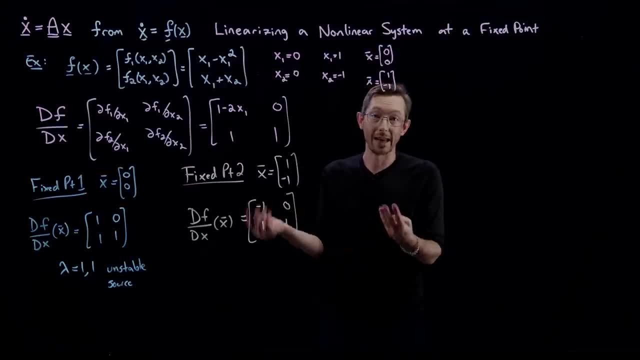 This is more interesting. Now. my eigenvalues are going to be saddle points. So I have 1 stable. you know, 1 lambda is plus 1, and 1 lambda is minus 1, so I get lambda plus or minus 1.. 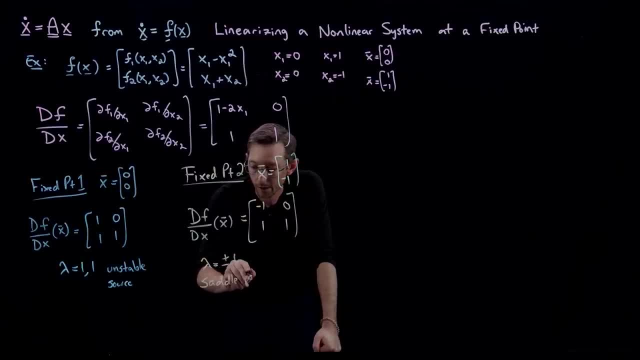 So this is a saddle point, Okay, which is kind of cool. And if I wanted to figure out what directions were stable and unstable, I'd find the eigenvectors of this. If I wanted to know the eigenvectors corresponding to the stable and unstable directions. 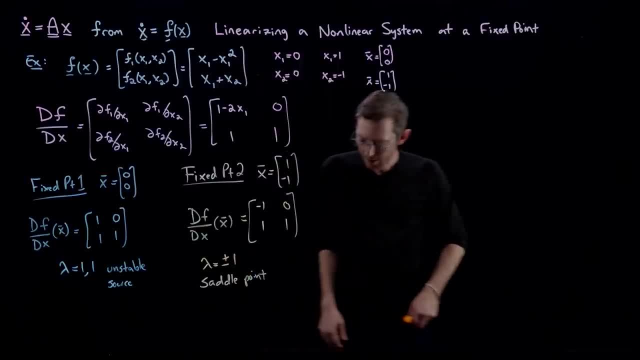 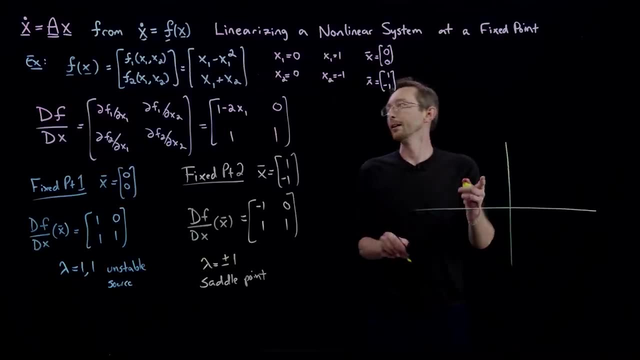 I'd find its eigenvectors similar for this, And I haven't done this in my notes, so I'm a little nervous about it, but I think it should be fine. So now, if I look in my, you know, x1, x2 plane, 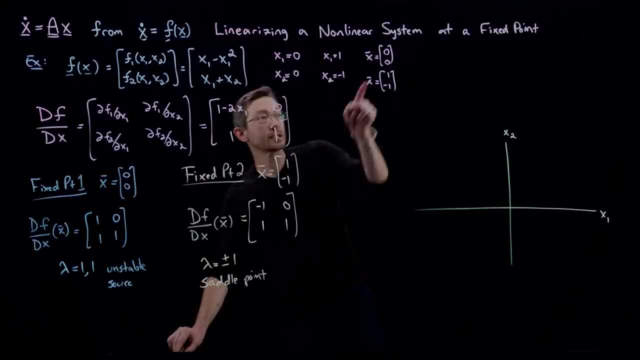 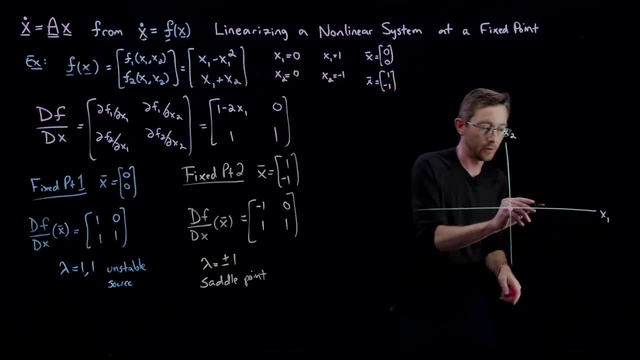 my phase plane. I have a fixed point 0, 0, right here, this fixed point right here, and I have another fixed point at 1, minus 1, 1, minus 1, down here, And we know that locally. 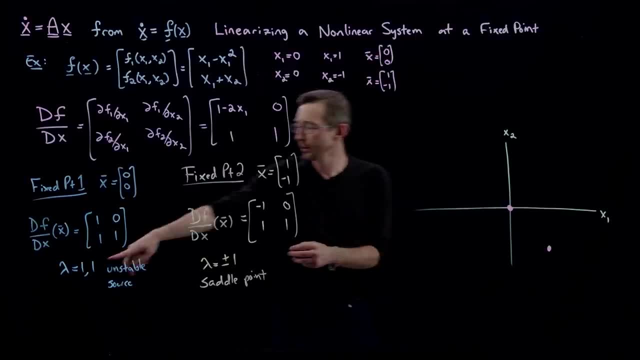 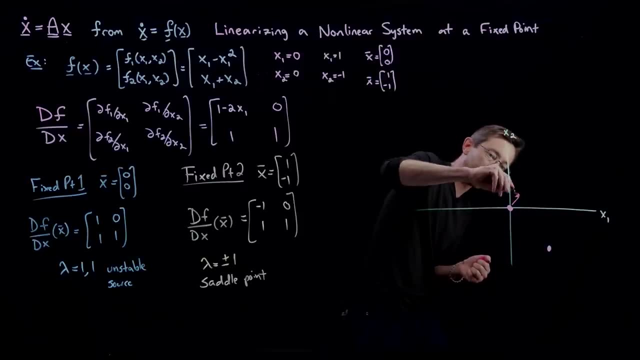 zoomed in locally to this point 0, 0,. my dynamics are unstable. It's an unstable source And because these eigenvalues are equal, I'm assuming it kind of is just like unstable the same magnitude in every direction. 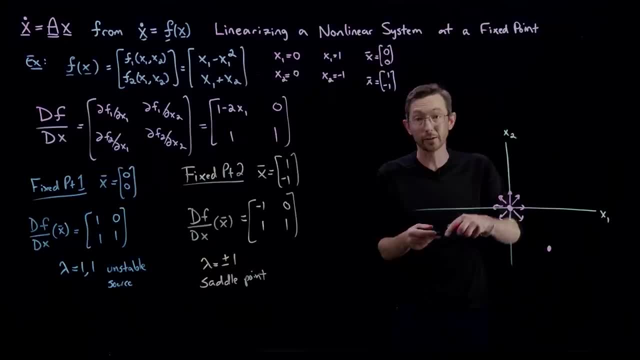 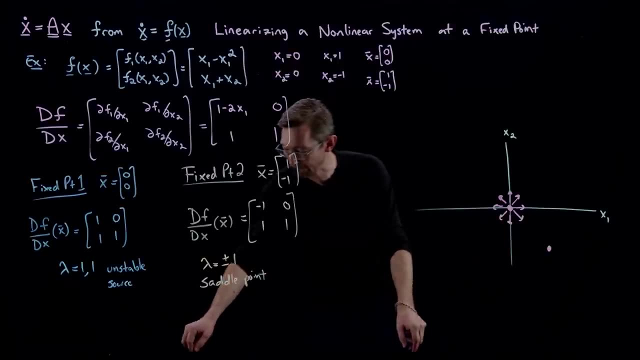 kind of like this: That is what this point locally linearly looks like, And this point is going to be a saddle point. okay, And so that point, locally linear- I don't know what directions are going to be stable and unstable, but it probably is going to have. 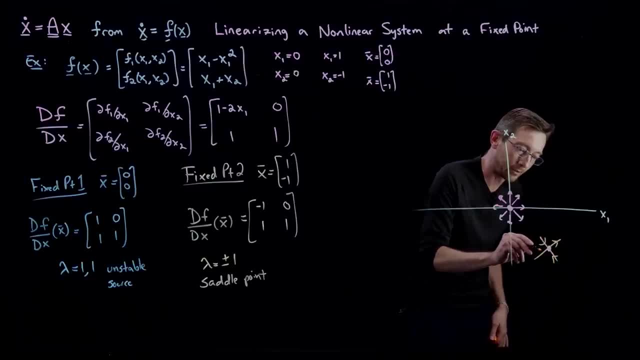 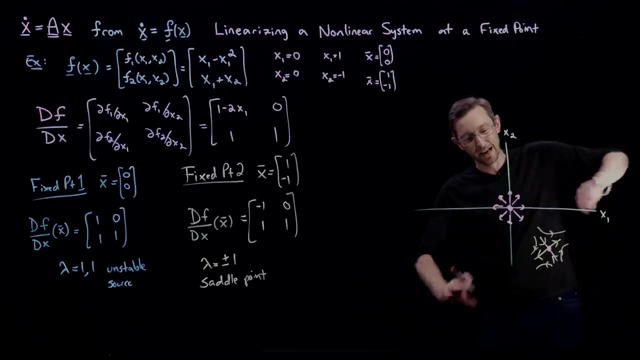 something like this, where these guys are locally stable and these guys are locally unstable And things kind of. I hope I drew this right. things kind of go in this orientation And who knows what happens between these? Probably something catastrophic, You know, I'm assuming what happens is that. 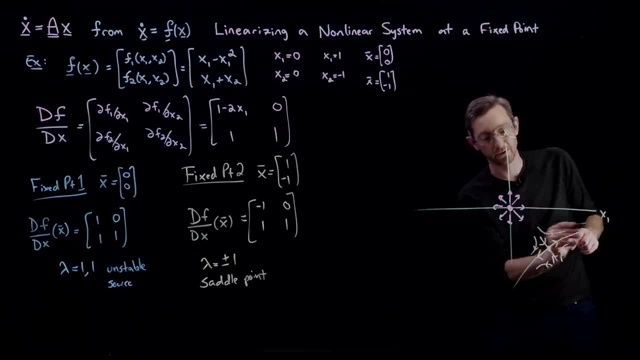 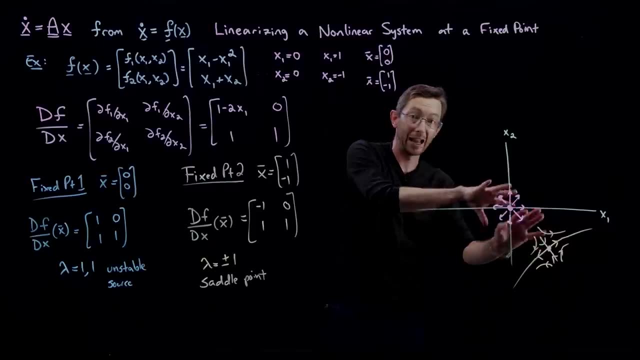 maybe you know, maybe there's some behavior here where these two meet. I don't know, That's something we'll talk about in another day- is: how do you interpolate or infer what happens between these fixed points With this linear analysis? 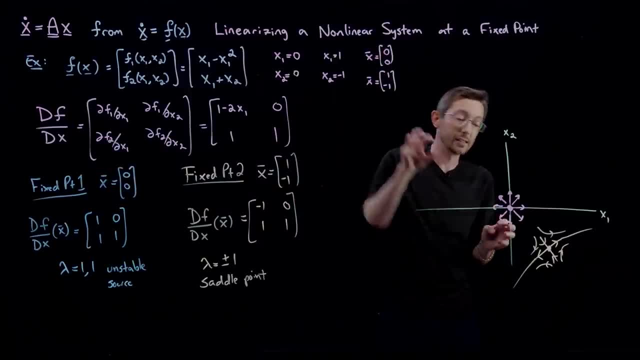 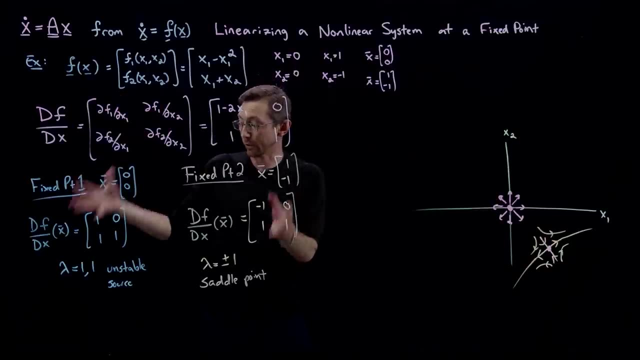 all that we can say is that there are these fixed points, and if we zoom in to a really small neighborhood, they behave linearly like X. dot equals AX according to these Jacobian A matrices. okay, So pretty cool that you can really start to analyze. 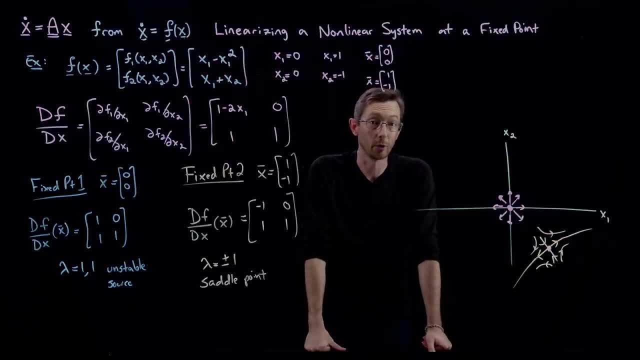 really nasty systems using these linear techniques that I showed you before And one of the ones you know I love doing. I'll show you this in another video. you can have things like you know. I have a saddle point here and maybe I have a spiral sink here. 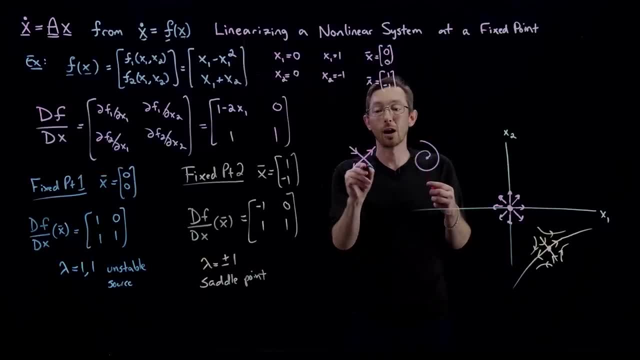 And so I can do things like infer. well, probably this will connect to that and you can actually start to complete this kind of global phase portrait. You know, you can start piecing together kind of globally what's gonna happen in some of these nonlinear systems. 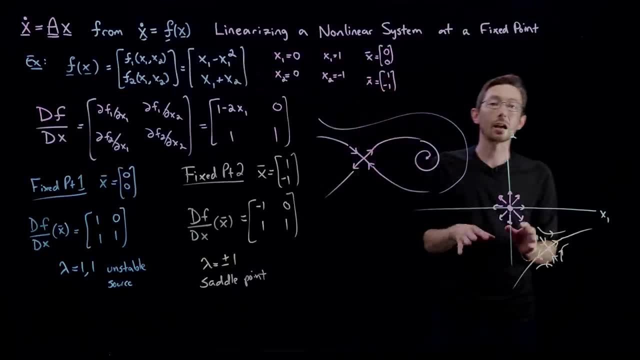 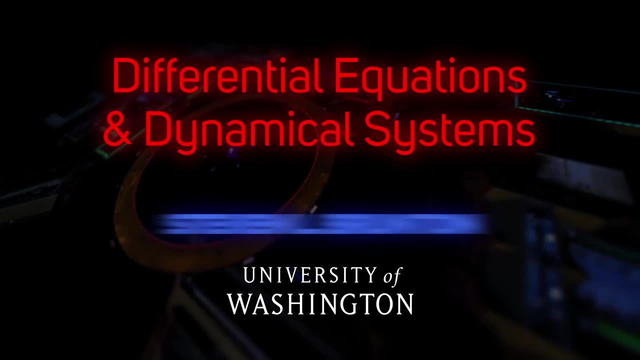 based on these rules and these linearizations. Okay, that's all coming up soon, so thank you very much, Thank you. 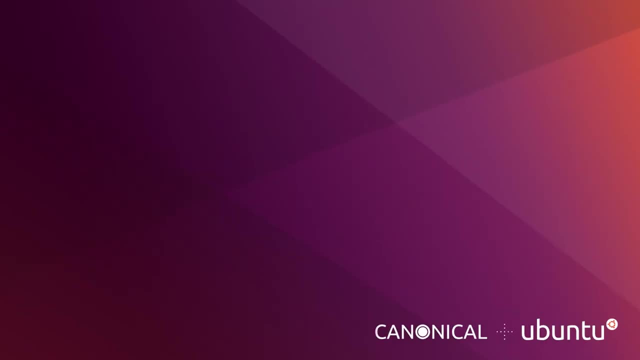 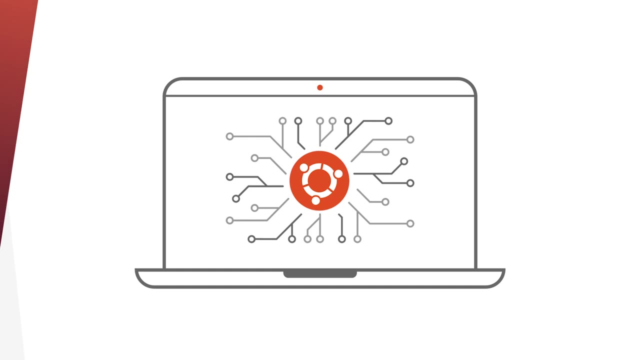 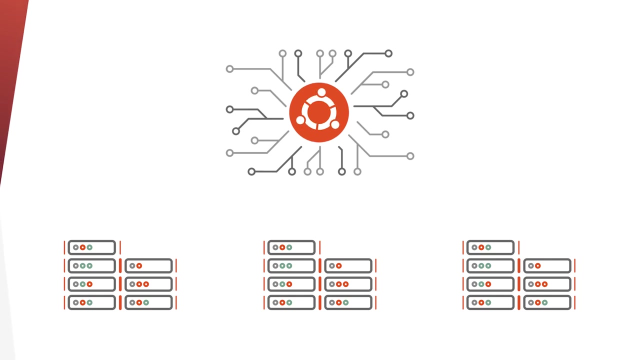 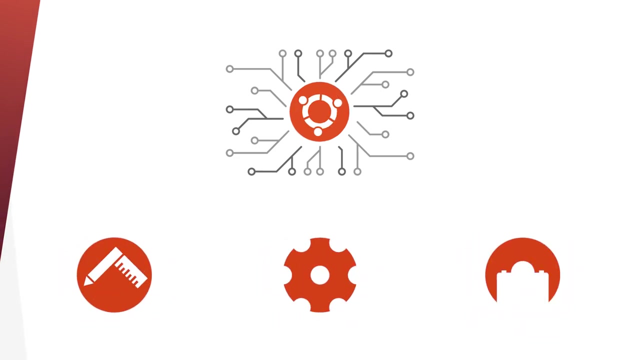 High performance computing uses supercomputers and computer clusters to solve advanced computational problems, Computational problems that require computing power and performance that is beyond the capabilities of a typical desktop computer or a workstation. These large computational problems exist in numerous fields, such as science, engineering or business. In the beginning, 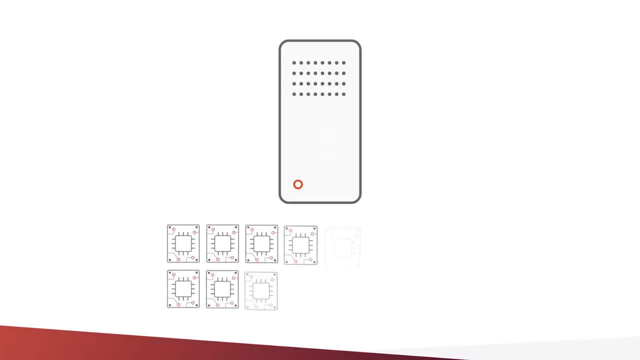 large and very expensive computers with multiple processors were built. They were called supercomputers. These supercomputers operated as a single system and worked to solve these large problems. This evolved over time to smaller, just as powerful computers with fewer and more specialized processors that shared their memory. They used fewer processors and